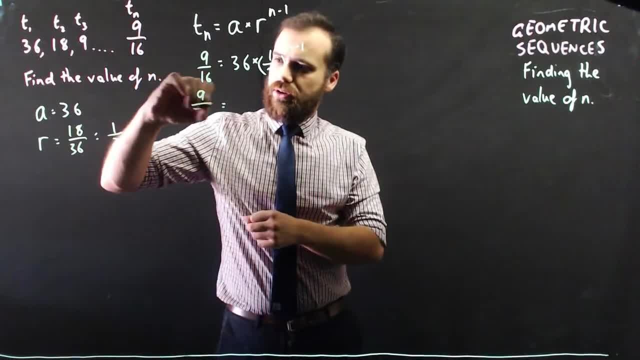 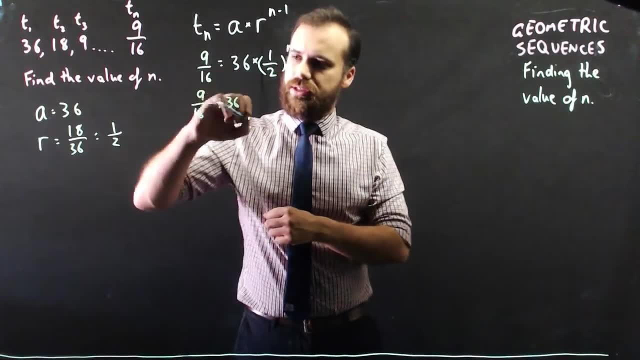 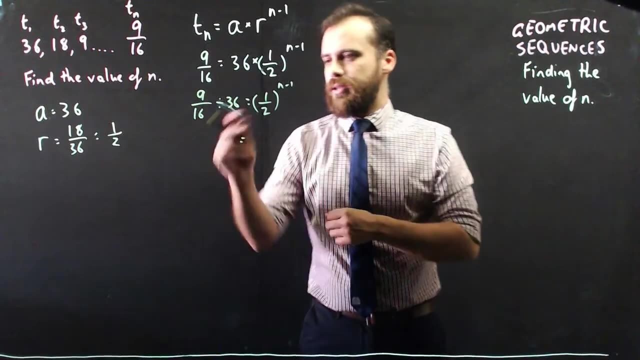 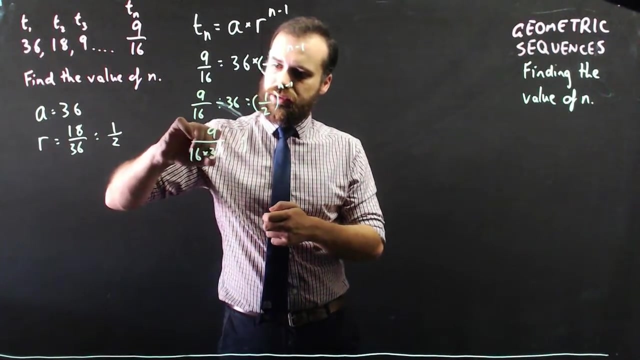 36 by dividing by 36.. So 9 on 16,. how should I write that? Divided by 36 equals 9 on 16.. So that's equal to 1 half n minus 1.. Now, really that's the same as 9 on 16 times 36.. 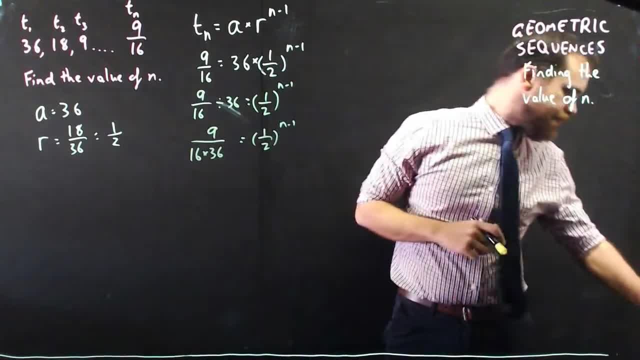 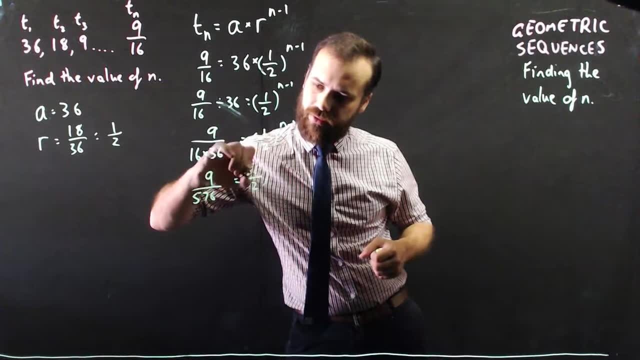 You might need a calculator for that. So that's going to be 9 on 576, which is equal to 1 half n minus 1. 9 on 576, what's the answer to that? Twitter На R-1.. 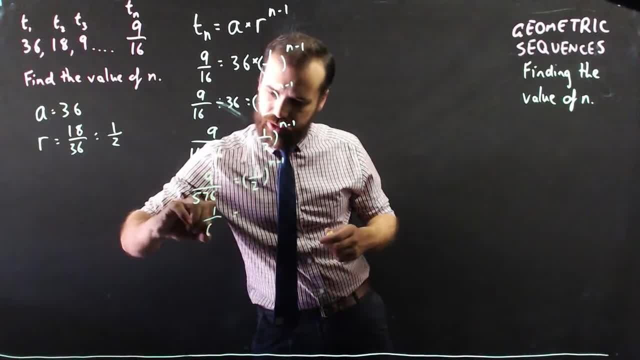 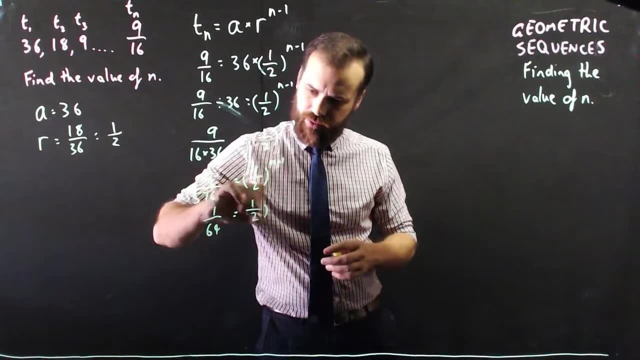 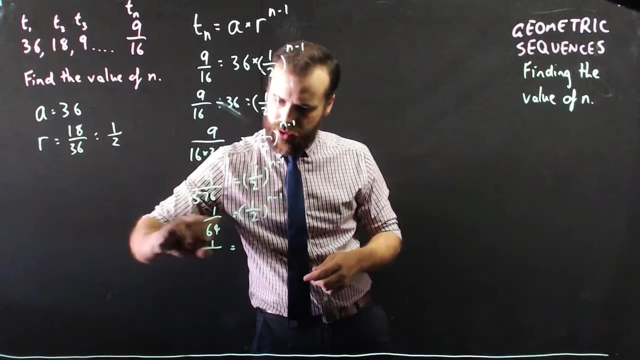 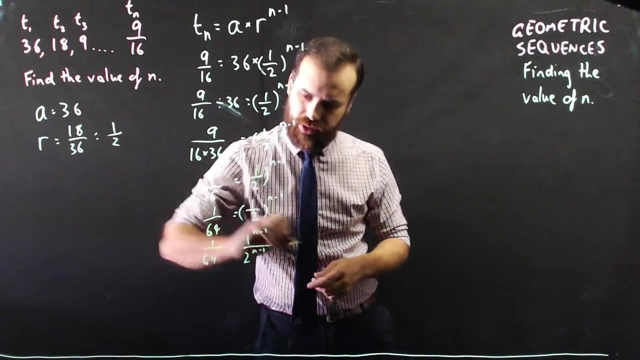 6 simplifies to 1 on 64.. Okay, getting there. 1 half n minus 1.. Now that's going to be the same as 1 on 64 equals 1 to the n minus 1 over 2 to the n minus 1.. Okay, so 1 raised. 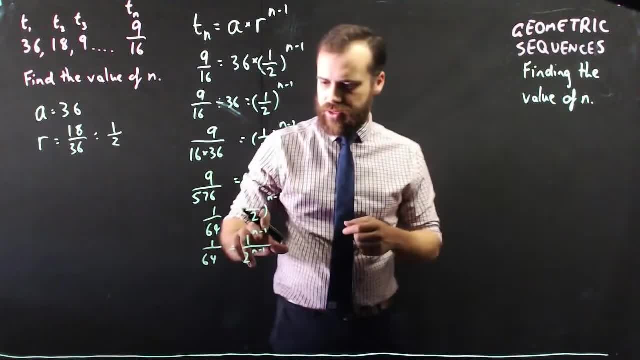 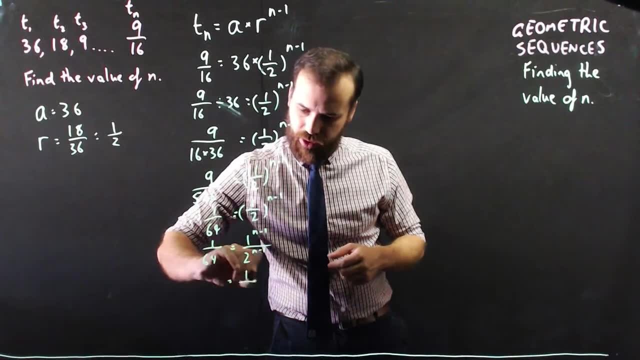 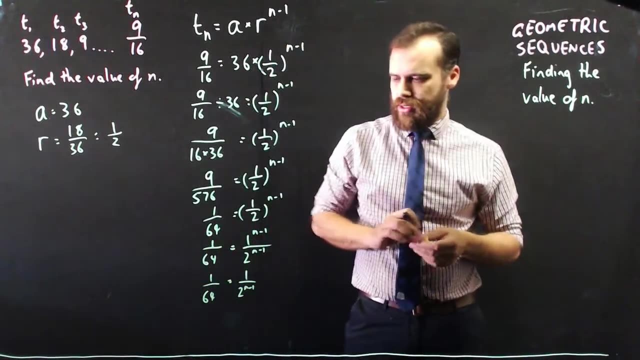 to the power of anything is going to be 1.. So we don't really need the n minus 1 here for the 1.. So we can just say that 1 over 2 to the n minus 1 equals 1 on 64.. Now here. 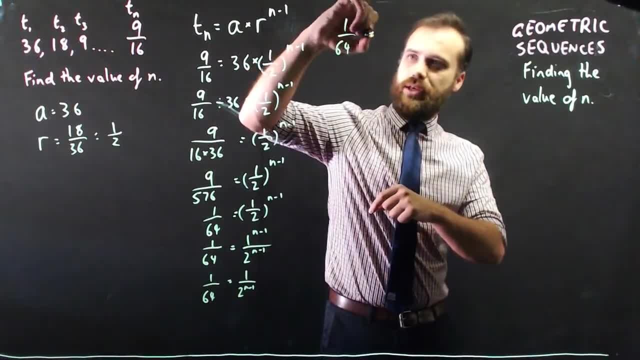 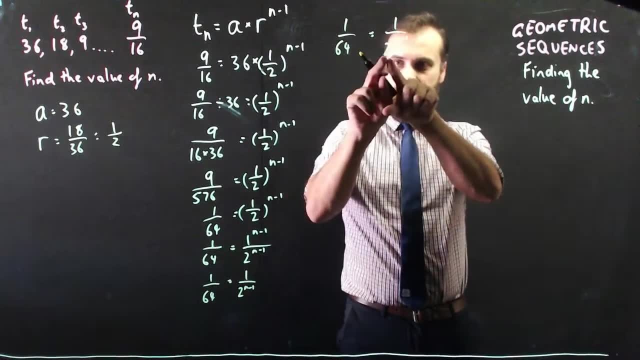 I'll just rewrite that 1 on 64 equals 1 on 2 to the n minus 1.. We could rewrite 64 as a power of 2. That's called equating the bases, and you've done that before. 1 on. 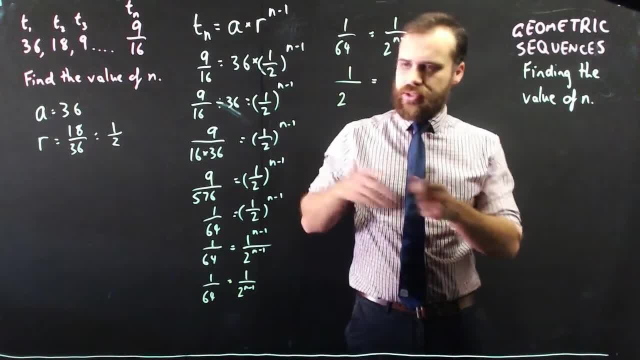 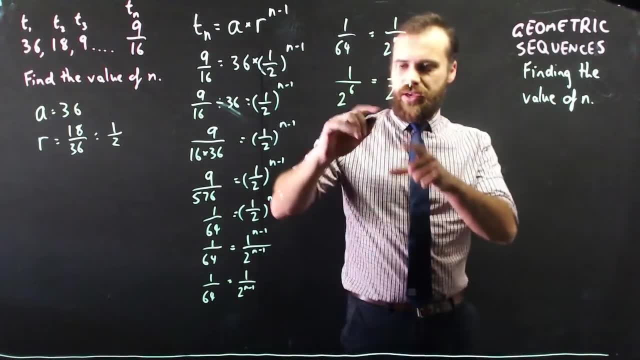 now 2 to the power of 2,, 4,, 8,, 16,, 32,, 64,. 2 to the power of 6 equals 1 on 2 to the power of n minus 1.. Therefore, if 1 on 2 to the power of 6 equals 1 on 2 to the power of n, 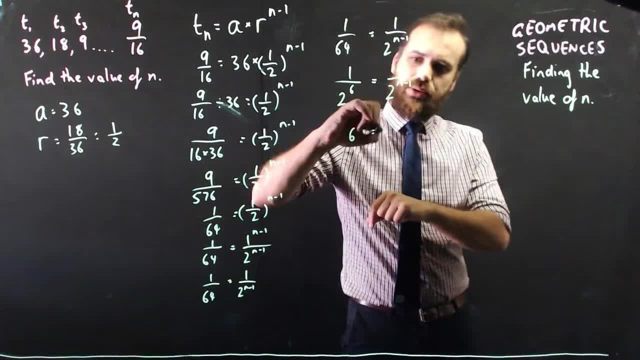 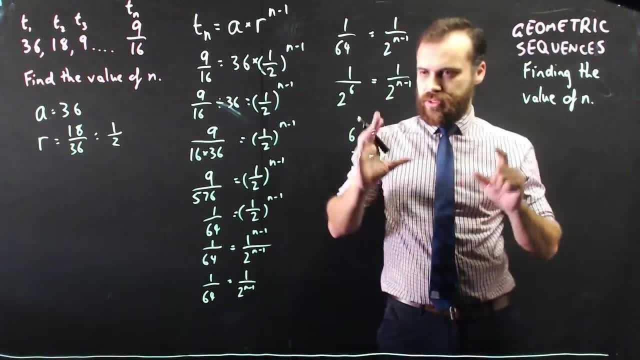 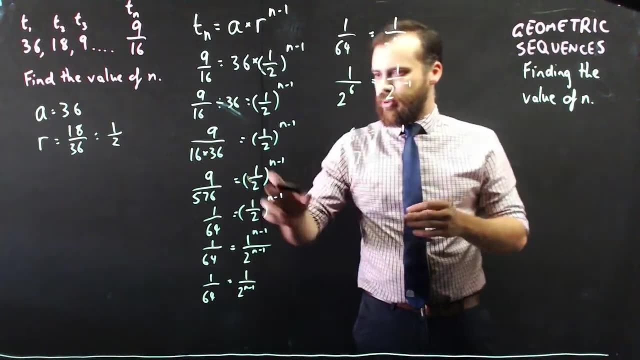 minus 1, then this must equal this, So 6 must equal n minus 1, which means that n equals 7.. Alright, that's a complicated question and there's a few little skills in there that you need. Probably the most important one there is that equating bases idea Just before.